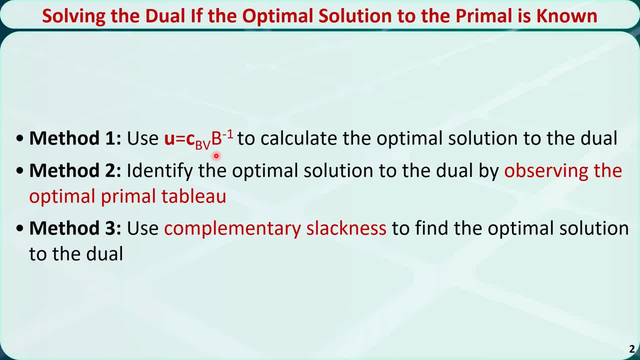 the optimal solution to the dual. Method 2, we can identify the optimal solution to the dual by observing the optimal primal tableau. Method 3, we can use complementary slackness to find the optimal solution to the dual. What if we don't know the optimal solution to the primal? 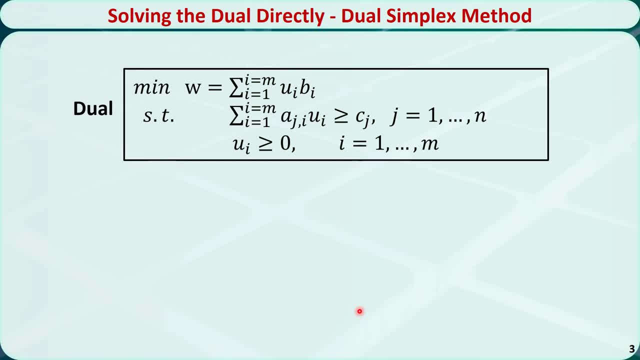 In that case we cannot use these three methods. We can use another method called the dual simplex method. The dual simplex method has three steps. In step 1, we need to reformulate the dual problem, so it will be a maximization problem. 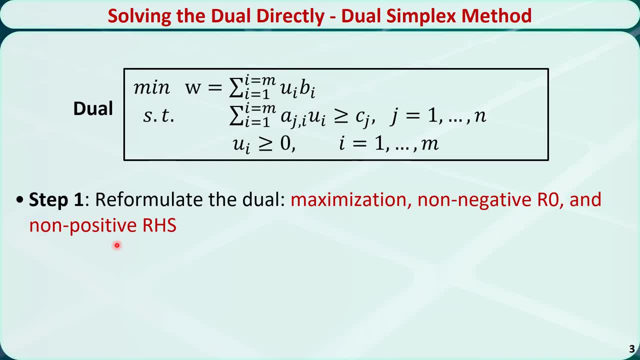 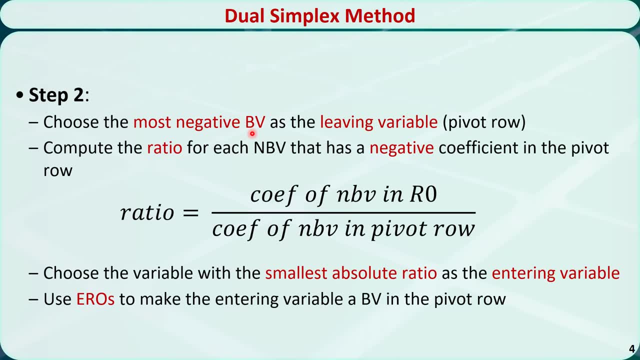 with non-negative root 0 and non-positive right-hand side RHS. In step 2, we need to choose the most negative basic variable as a living variable and the row will be the pivot row, Then compute the ratio for each non-basic variable that has a negative coefficient in. 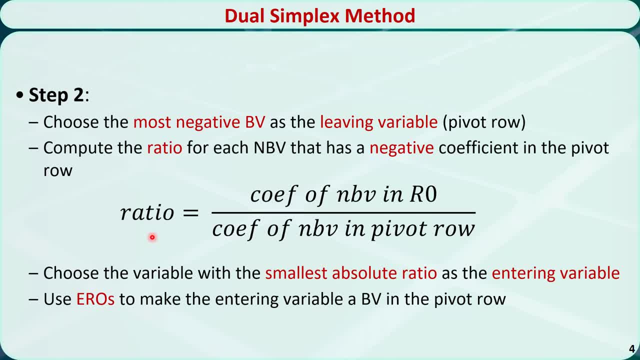 the pivot row. The ratio is the coefficient of a non-basic variable in row 0 over the coefficient of the non-basic variable in the pivot row. After that, we choose the variable with the smallest absolute ratio as the entering variable. We use elementary row operations, or EROs, to make the entering variable a basic variable. 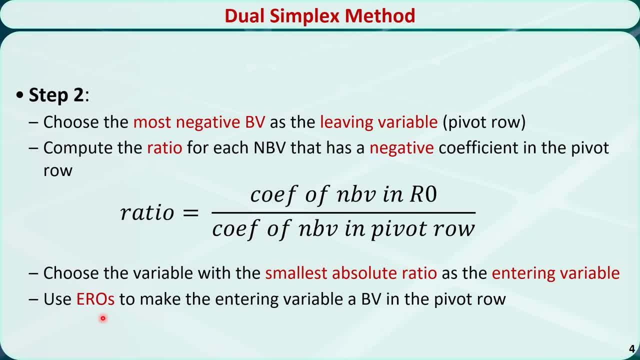 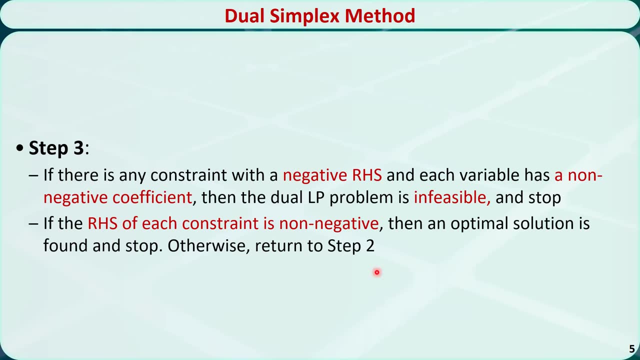 in the pivot row. In the dual simplex method we determine the living variable first, then the entering variable, which is quite different from the regular or primal simplex method. In step 3, if there is any constraint with a negative right-hand side, and each variable. 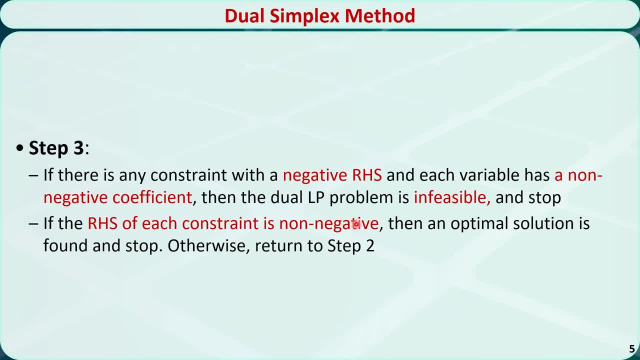 has a non-negative coefficient, then the dual linear programming problem is infeasible. If the right-hand side of each constraint is non-negative, then an optimum solution is found and stop. Otherwise return to step 2.. Let's illustrate the dual simplex method using this example. 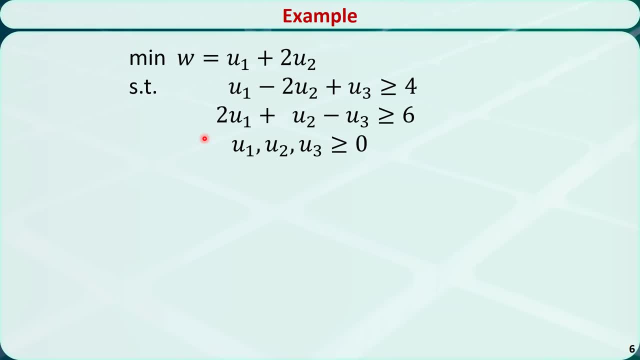 This is a dual problem in the standard form. It's a minimization problem. All the constraints are greater than or equal to the right-hand side. All the variables are greater than or equal to 0.. The first step of the dual simplex method is to reformulate the dual problem. 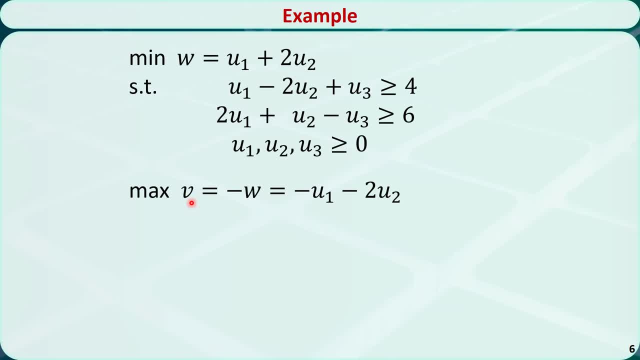 We change this problem to a maximization problem by taking the opposite of the objective function and give it to v. In the canonical form, each variable has a non-negative coefficient in row 0. We need to introduce two excess variables- e1 and e2, to make these two equality constraints. Now the right-hand side of both constraints. 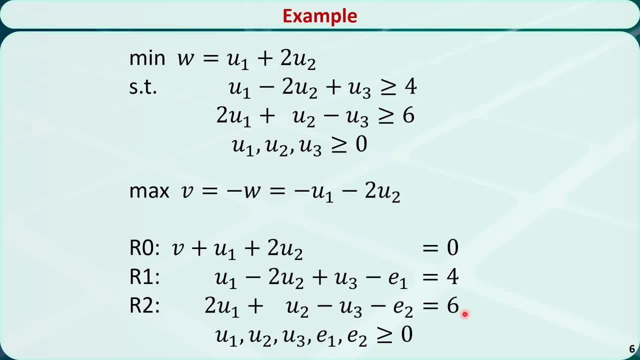 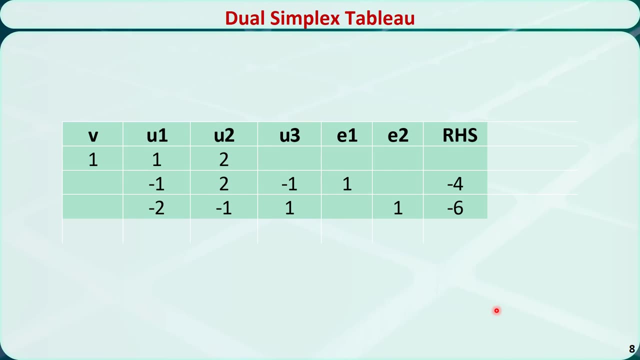 is positive, We need to make them non-positive By multiplying negative 1 for both sides. This is the updated canonical form. Let's write this in a tableau. Now let's find the basic variables. They are the variables with the coefficient 1 and appear in only one row and not other rows. So the 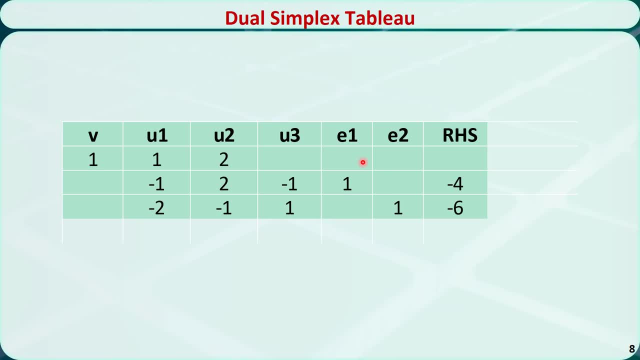 basic variables are e1 and e2.. Remember, v is not a basic variable. It represents the objective function value, but by convention we just put it in this column. All other variables are non-basic variables. Let's set the non-basic variables to 0 and. 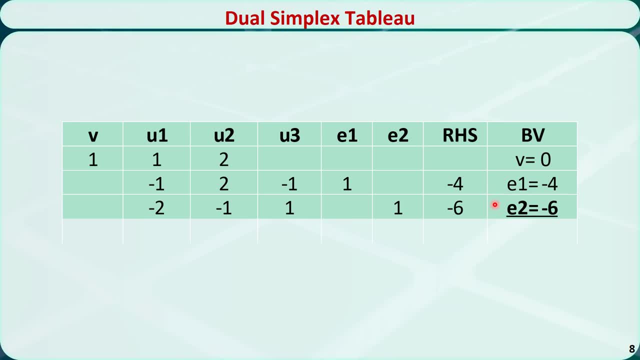 solve for the basic variables. This is what we get. Now we need to check if this tableau is optimal or not. by checking if the right-hand side of each constraint is non-negative, We find that the right-hand side of both constraints are negative, so it's not optimal yet. 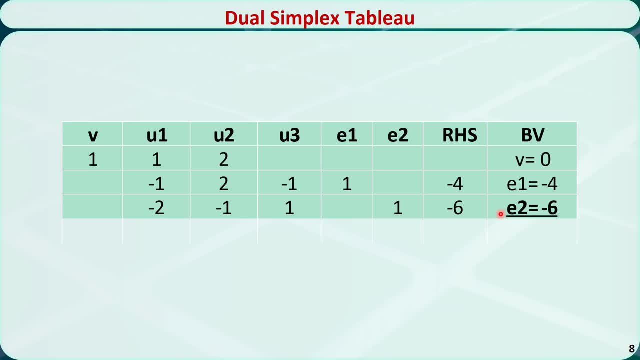 We need to choose the most negative basic variable as the leaving variable, which is e2, and this row will be the pivot row. Let's compute the ratio for each non-basic variable that has a negative coefficient in the pivot row. The ratio is the coefficient of a non-basic. 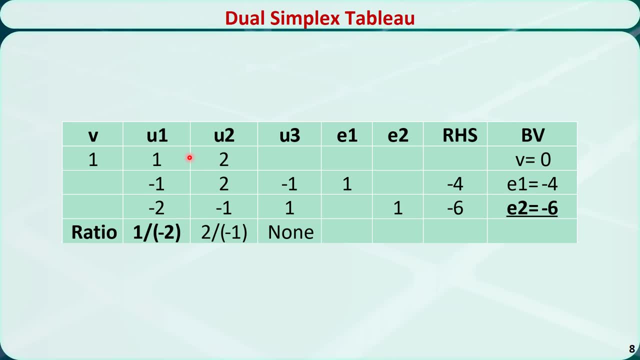 variable in row 0 over the coefficient of that non-basic variable in the pivot row. 1 divided by negative, Negative 2 is negative 1 over 2.. 2 divided by negative 1 is negative 2.. After that we choose the variable with the smallest absolute ratio as the entering variable. 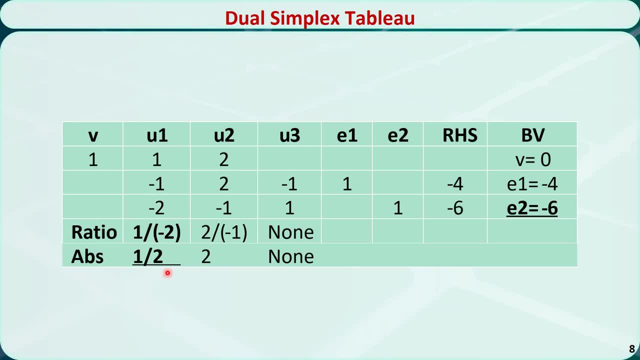 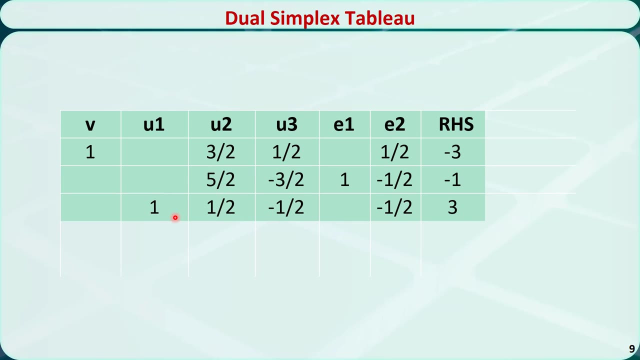 which is u1.. We use EROs to make this entering variable have a coefficient 1 in the pivot row and make it disappear in all other rows. This is the new tableau. Let's solve for the basic variables. There are u1 and u1.. 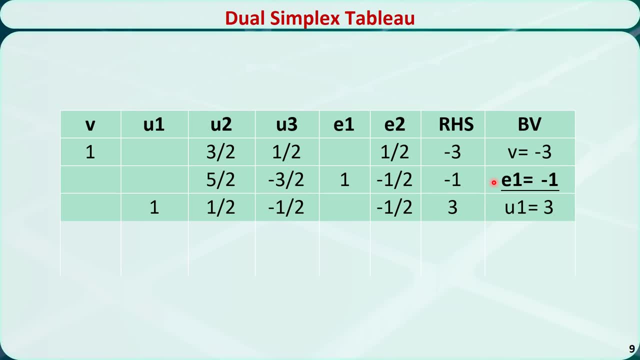 Now we need to check if the tableau is optimal or not. by checking if the right-hand side of each constraint is non-negative, We find that the right-hand side of this constraint is still negative, so it's not optimal. yet We need to choose the most negative basic variable as the leaving variable, which is: 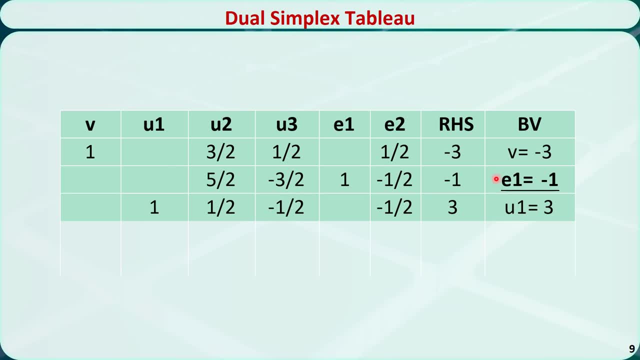 u1, and this row will be the pivot row. Let's solve for the basic variables. There are e1 and u1.. Let's solve for the basic variables: There are e1 and u1.. Let's compute the ratio for each non-basic variable that has a negative coefficient in. 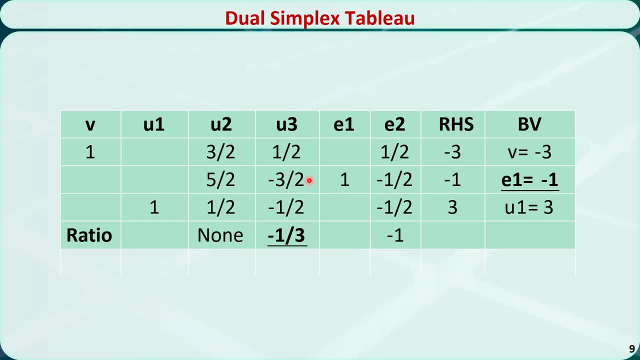 the pivot row. The ratio is the coefficient of a non-basic variable in row 0 over the coefficient of that non-basic variable in the pivot row 1 over 2, divided by negative 3 over 2 is negative 1 over 3.. 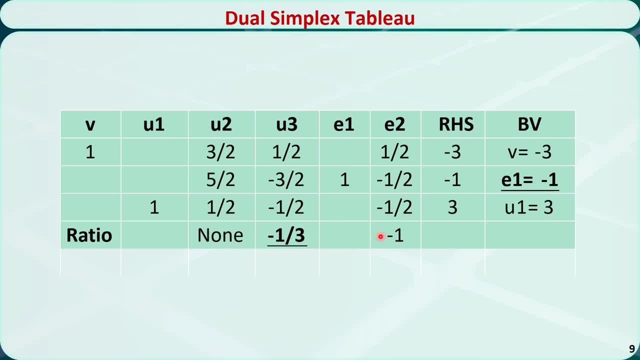 1 over 2, divided by negative 1 over 2 is negative 1.. After that, we choose the variable with the smallest absolute ratio as the entering variable, which is u3. We use ROs to make this entering variable have a coefficient 1 in the pivot row and make it disappear in all other rows. 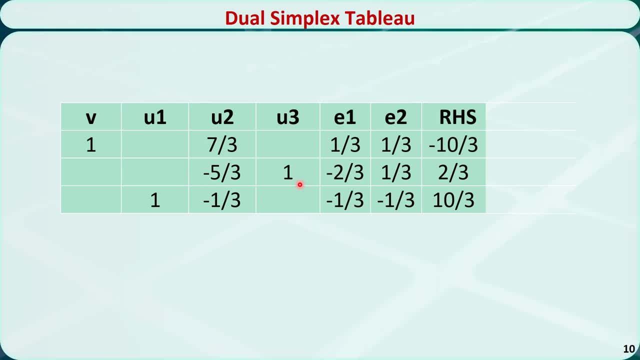 This is the new tableau. Now let's solve for the basic variables. There are u3 and u1.. Now we need to check if this tableau is optimal or not by checking if the right-hand side of each constraint is non-negative. They are. 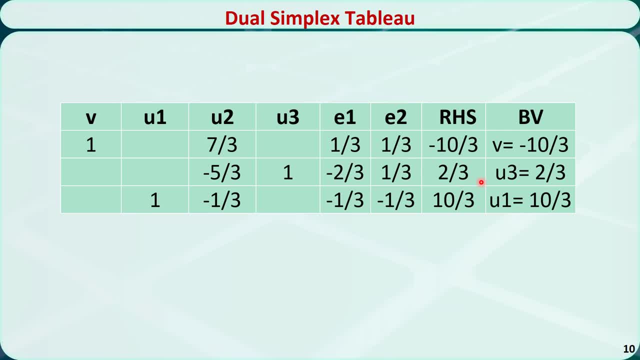 both positive. So this tableau is optimal. The optimal solution to the dual problem is: w is equal to negative, v is equal to 10 over 3.. u1 is equal to 10 over 3.. u3 is equal to 2 over 3.. 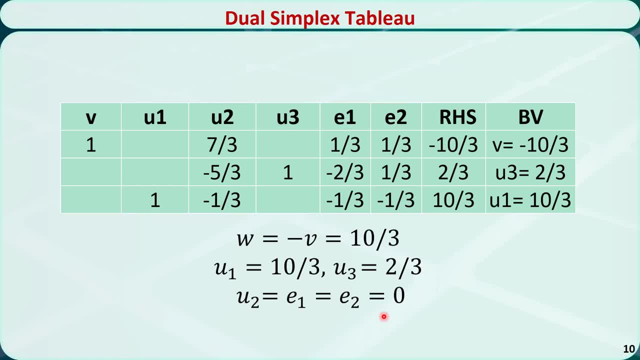 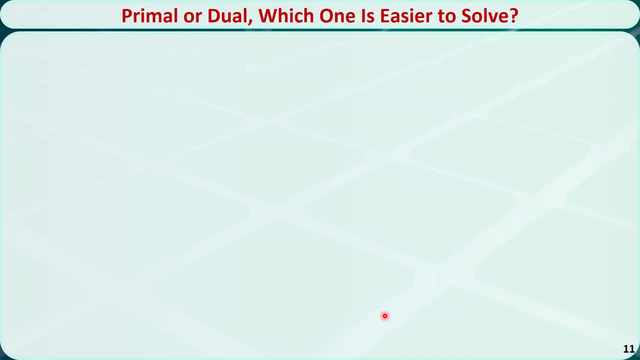 u2,, u1, and u2 are 0.. Now we know that each linear programming problem can be formulated from two perspectives: primal and dual. We can solve the primal using the primal simplex method and solve the dual using the dual simplex method. The question is, when should we solve the primal and when should we solve?